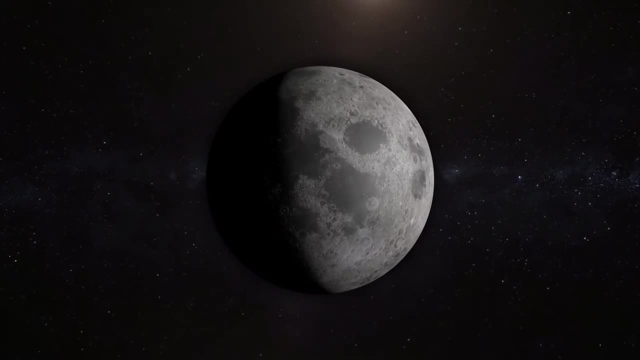 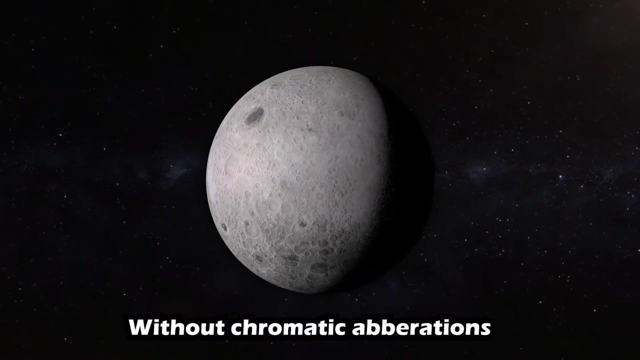 are truly grab-and-go telescopes. The only disadvantage of the refractor telescope is chromatic aberrations. When this chromatic aberration happens, instead of a sharp image, the image looks like this, which can be overcome by adding one more lens. This combination: 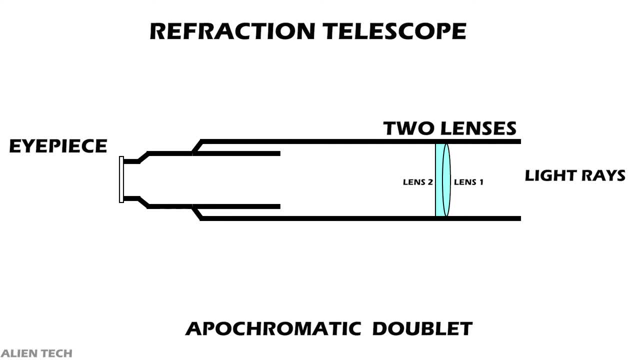 is known as apochromatic doublet. You can still get super-sharp images, but it is still a simple way to get the best perspective on any aspect. To correct this, a third lens is added. This type of telescope is called an aberachromatic. 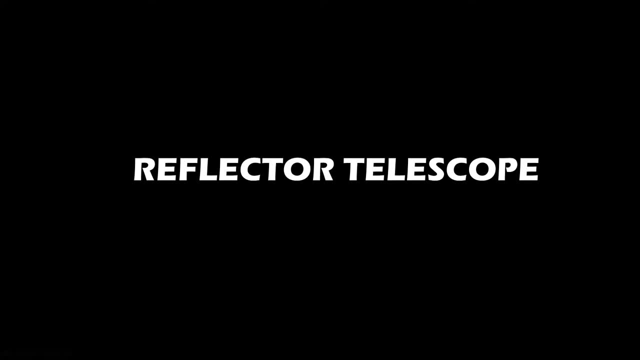 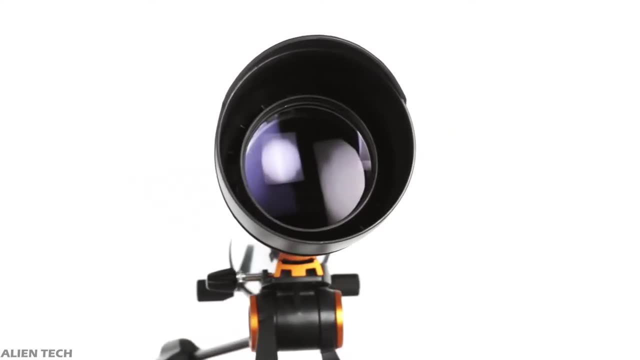 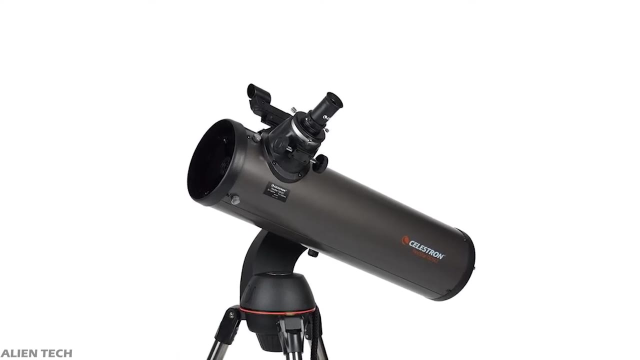 triplet. The second type of telescope is a reflector telescope. One of the biggest problems with the refractor telescope is that the cost for a bigger aperture is too much, So this problem is solved by reflector telescopes. These telescopes use a mirror to gather and focus light. The 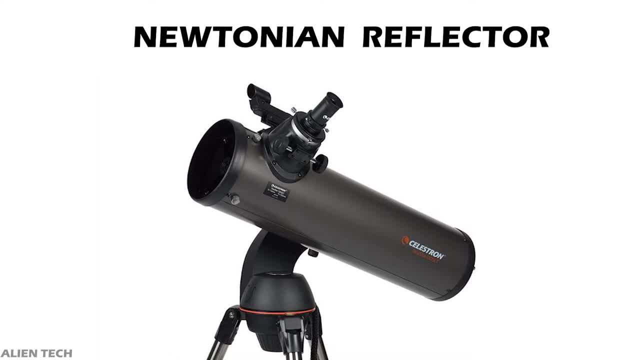 most common reflector we know is the Newtonian reflector. Newtonian reflector can only be used for five seconds. It is called a Newtonian reflector. Newtonian reflector is an elastic reflector. Their contrast is so strong that even light can easily be scratched by light. 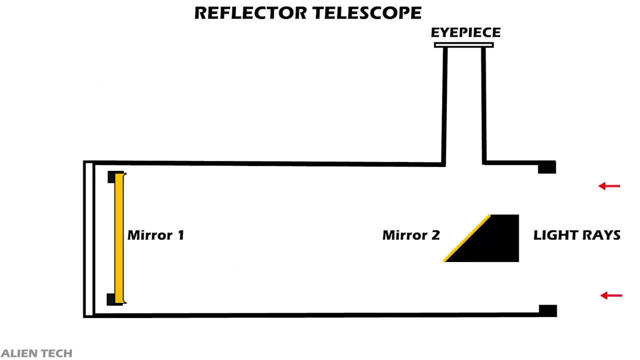 so It can easily 2 times as much as light Every single observable object in the near future reflector. because it was invented by Sir Isaac Newton, This type of telescope has a slightly curved concave mirror at the bottom of the tube which collects light. The collected light is 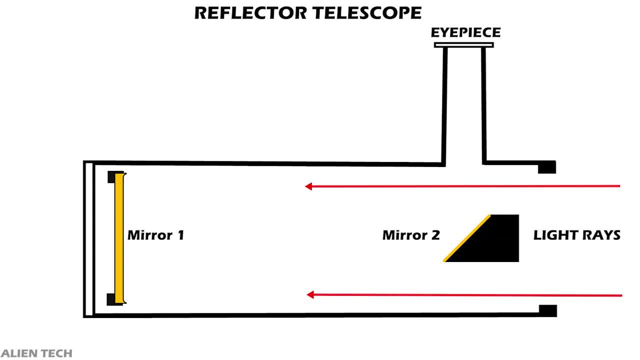 reflected to the top, where a secondary mirror directs this light to an eyepiece. One of the most important parts of the telescope is its aperture, and if you want the biggest aperture for the money you spend, then the reflector is the telescope. you should go for One of the most. 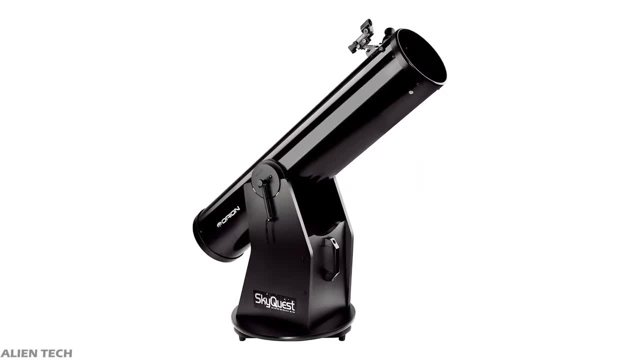 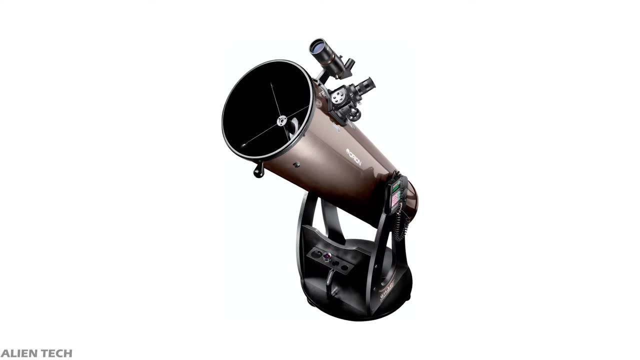 common reflector telescope types you'll find is a Domson-Yen telescope. These telescopes give excellent performance for the price you pay for. The refractor telescope does not need any collimation or adjustment. However, you'll need to collimate the reflector telescope once in a while. 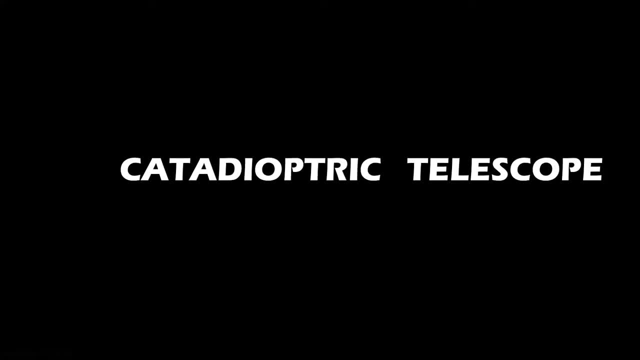 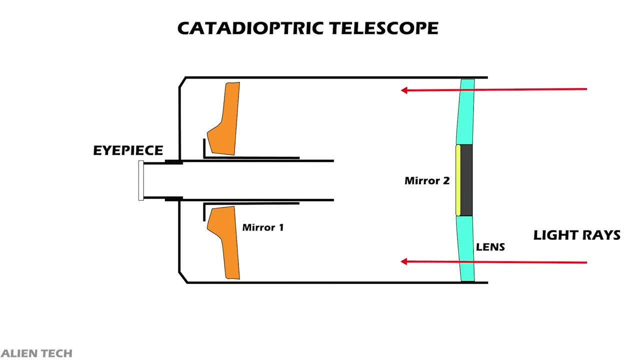 The third type of telescope is the catadioptric telescope. Catadioptric is a branch of optics where you deal with mirrors and lenses at the same time. So all the catadioptric telescope use the best of the refractor and the reflector telescope to form an image. That's why it's called. 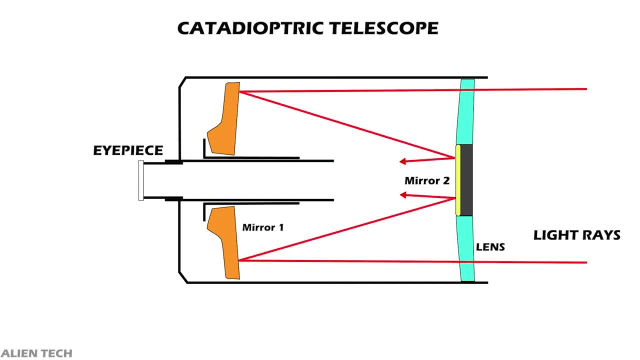 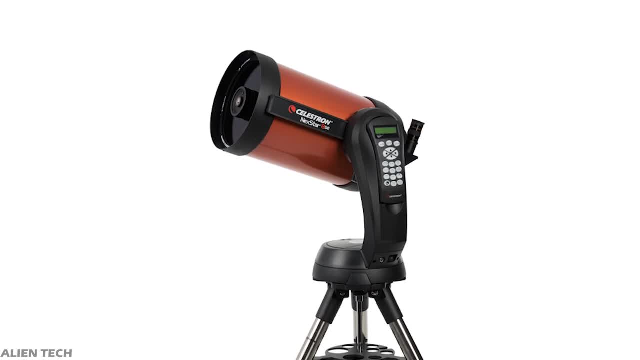 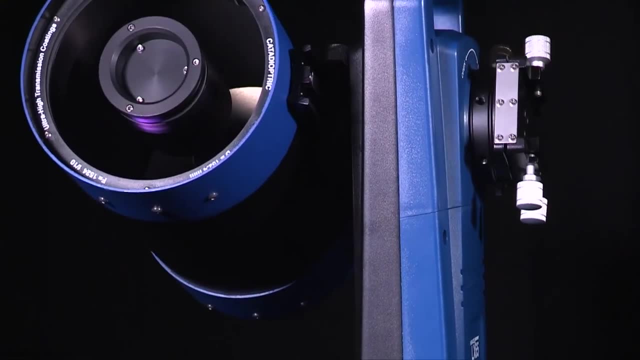 a compound or catadioptric telescope. The biggest plus point of these telescopes is that they are compact and lightweight. The telescopes which come under these categories are Schmidt-Cassegrain or Maxitoff-Cassegrain type telescopes. As these telescopes are compact, they're lightweight Because of this.